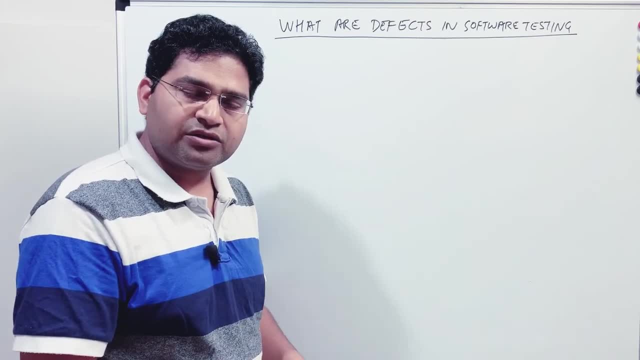 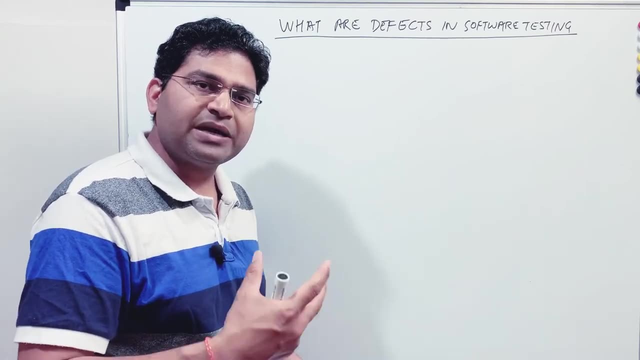 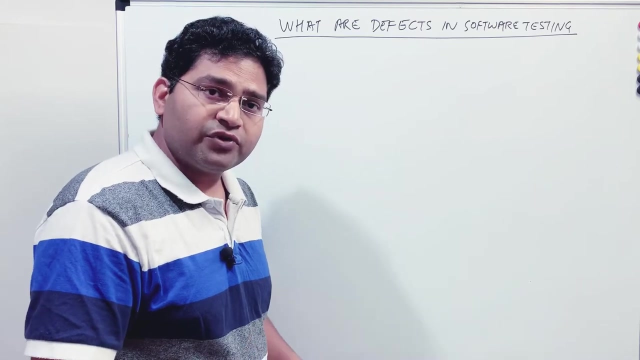 There is a design being made by the tech architects and all After that design, that design is implemented or the coding is done by the developers. Once the code is being packaged and deployed, that's when tester will actually launch the application or the software and start the verification process or the testing process right and 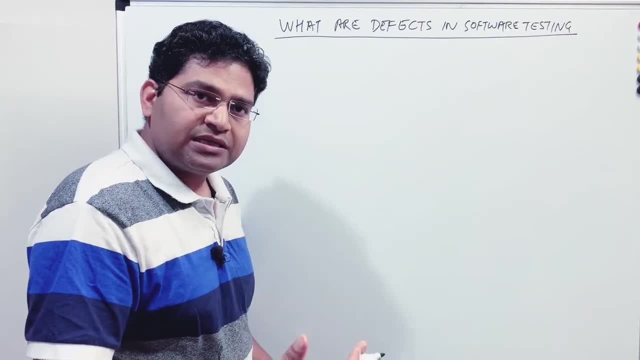 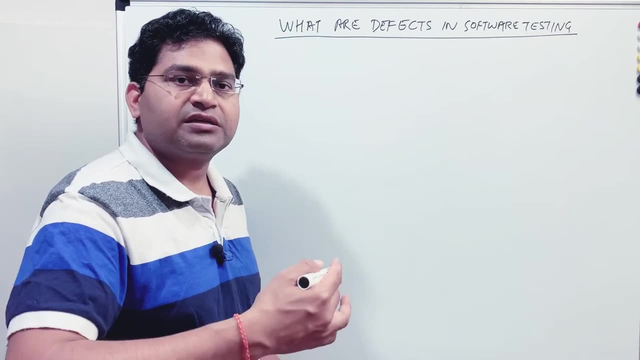 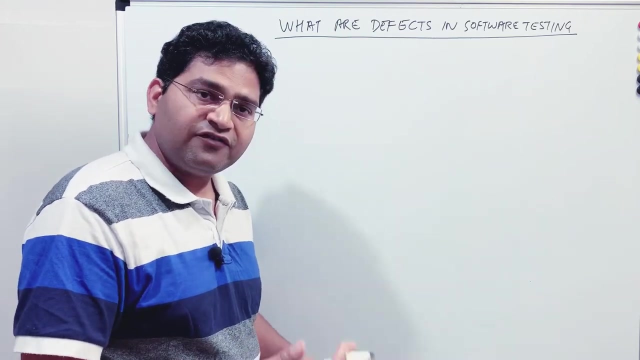 when he is doing the testing, he or she is doing the testing. if, If the expected result, or the actual result basically for a particular test case or scenario is not as expected, then that deviation is Known as defect or bug in the software. Okay, so it is very simple. 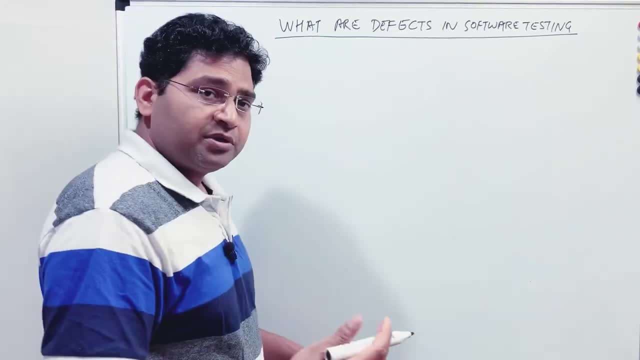 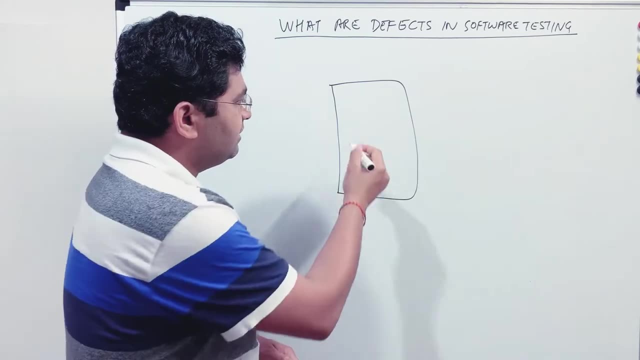 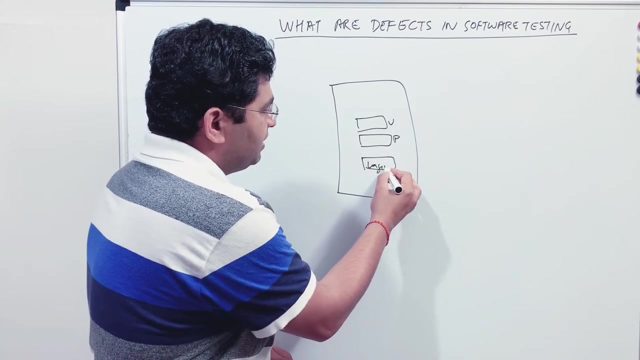 Say, for example- I'll take an example to explain this to you. So, for example, we have been taking the e-commerce website example. now on the e-commerce website, I Want to log in Using the username and password and click on login button right. So this is the login button. 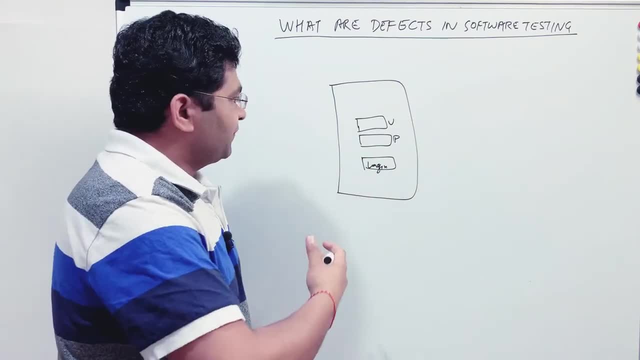 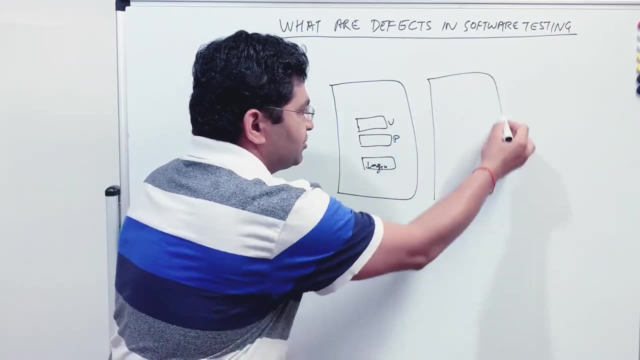 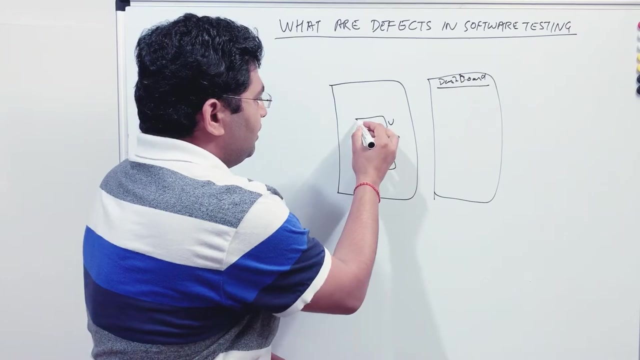 so I Have a test case which says when I use the valid username and password and click on login button, I should be redirected to the dashboard page, right. so dashboard Now. as Part of the test case, I have provided valid username, valid password and clicked on login button. 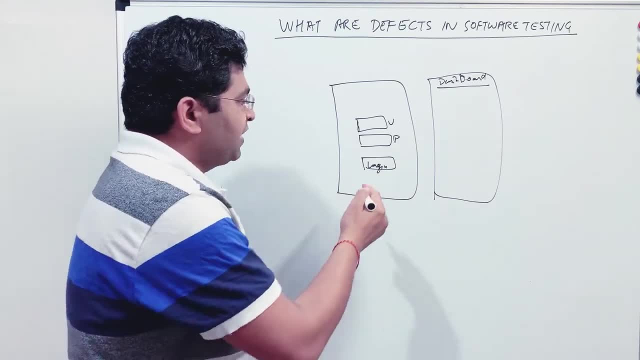 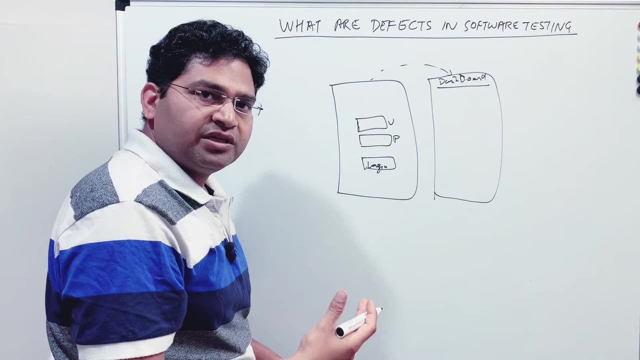 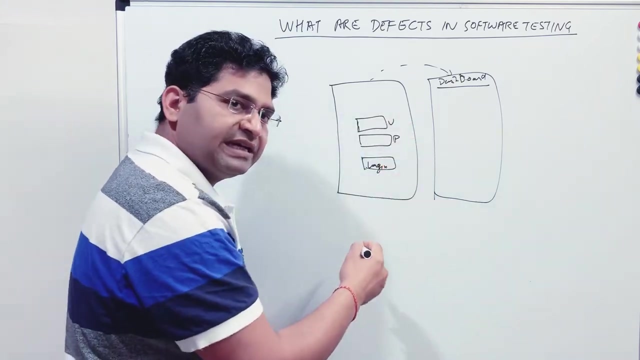 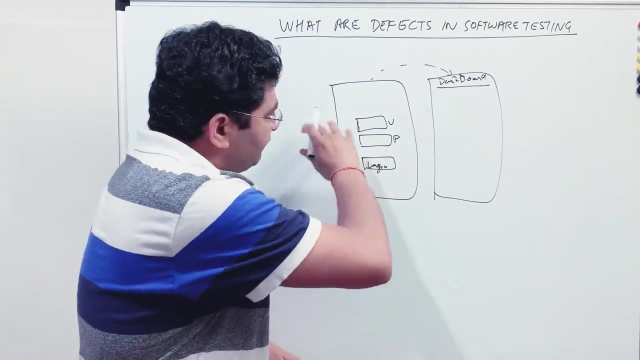 But once I click on login button, I am not redirected to this particular page, right to the dashboard page. what happens actually in the test environment is I, Once I click on the login button, this page, the login screen, get refreshed, Username, password disappear and I'm still on this login page, Okay. so if this is the case, 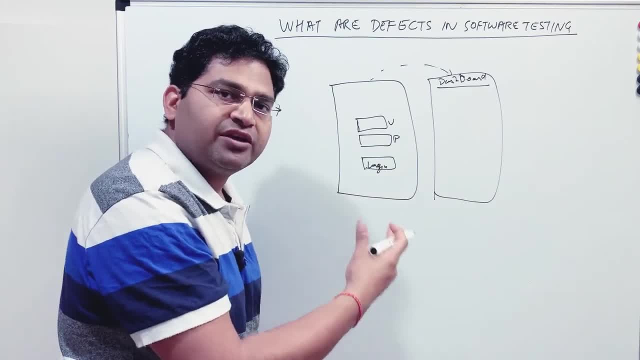 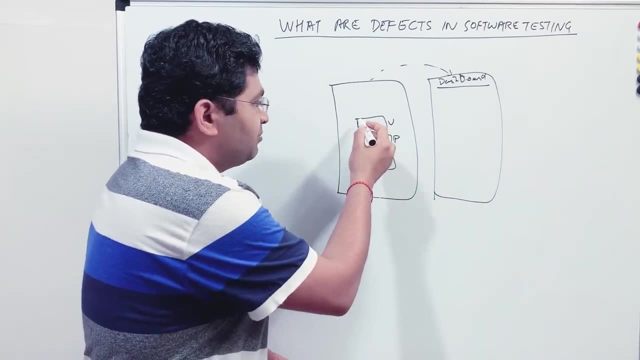 This is not what is the expected behavior of the test Right? So what, as a tester, I'll do is: I'll try to verify, I'll make sure that the username and password that I am using is correct. I'll try to analyze the logs and 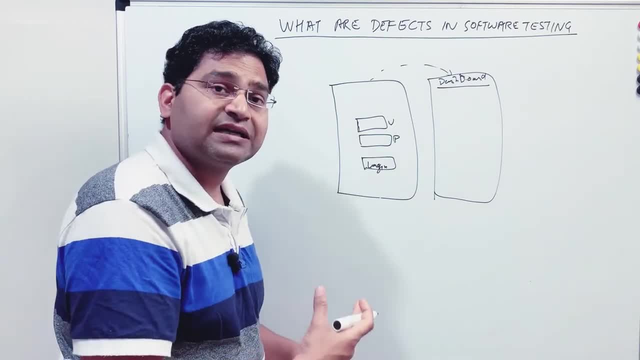 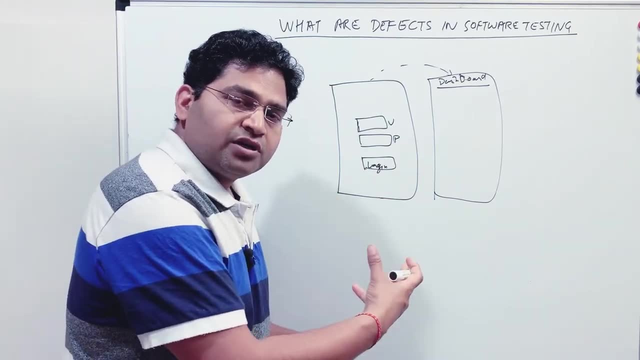 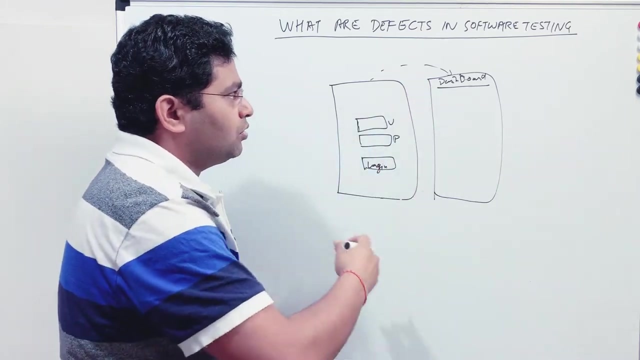 I'll try to analyze the browser logs and see what exactly the error is. Once I'm satisfied that the error is actually some sort of Configuration error or the coding error in that particular case, I'll raise that issue or the problem into the defect management tool. and that is what is. 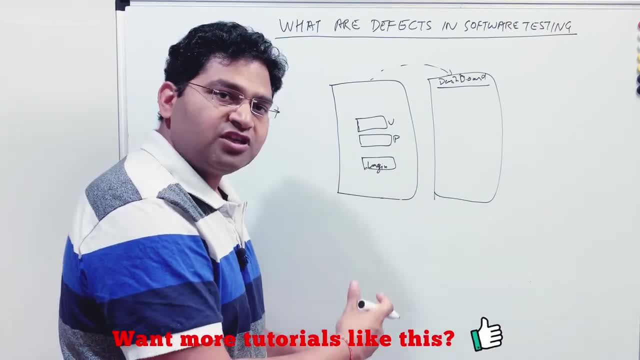 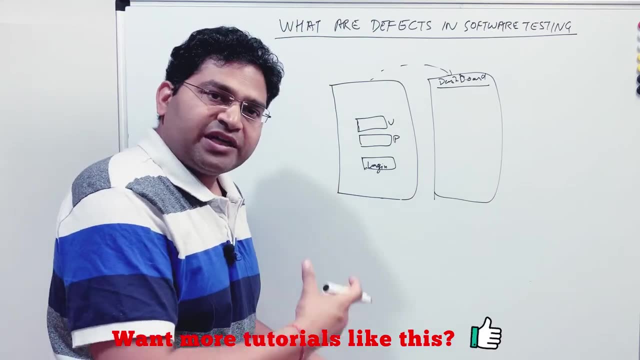 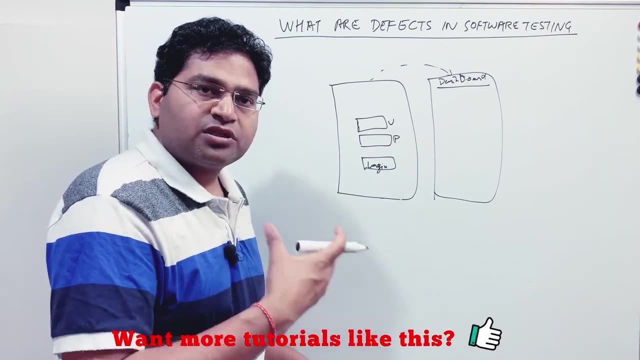 Defect or bug, or that is what is known as defect or bug in the software testing right. So any deviation From the expected outcome is a defect in software testing. Okay, so it can be at any level, So say, for example, in the software testing lifecycle, I am doing the functional testing. 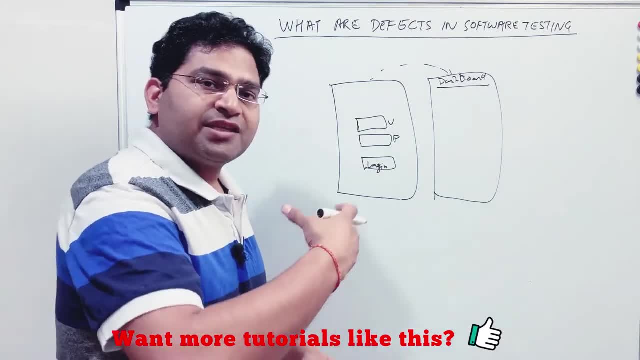 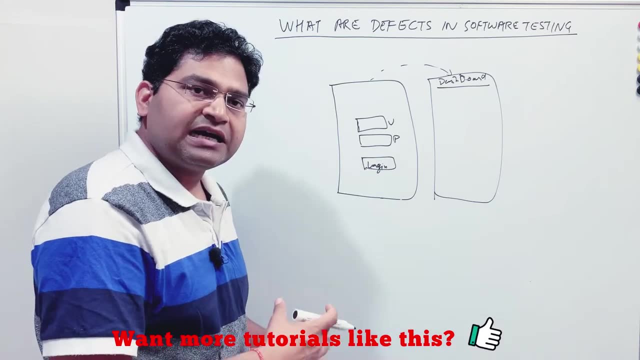 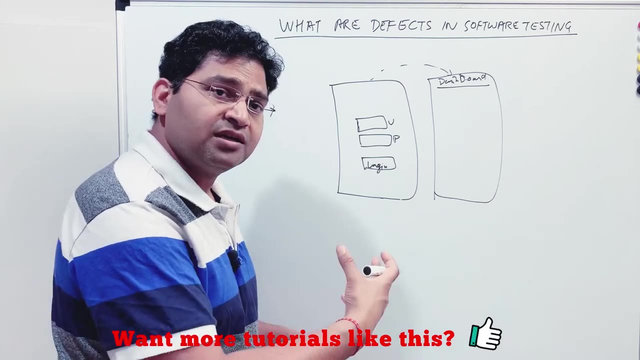 I can find defect in that Once I am into the Excel testing phase. there will be defects on that Even after the production deployment. if the customer finds that whatever he is looking for into the software his results are not as expected as he mentioned in the requirement, then that deviation is also a defect and needs to be raised. 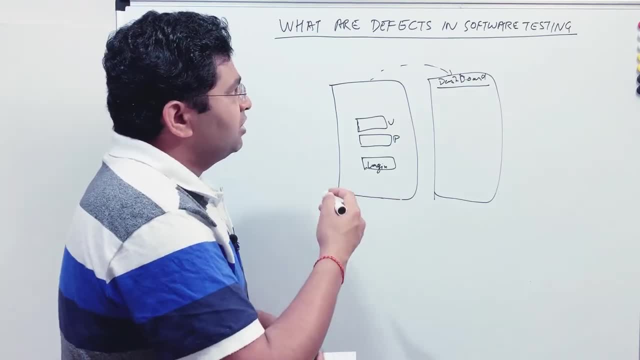 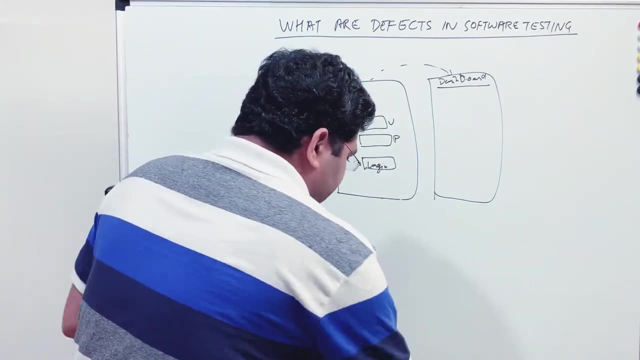 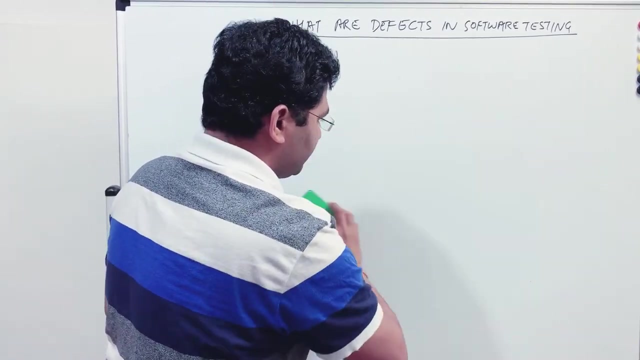 and fixed in the software right. So this is a brief definition of the defect or bug in software testing. Now there are a couple of key things or key metrics that you need to remember about the defects. So whenever you're doing software testing, some of the key metrics that you need to: 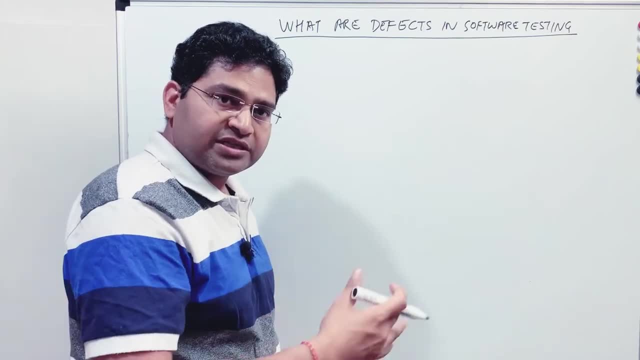 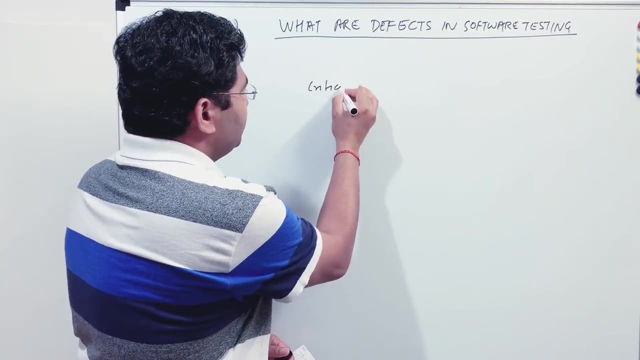 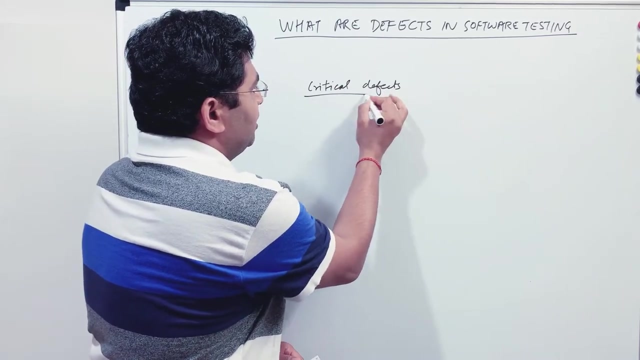 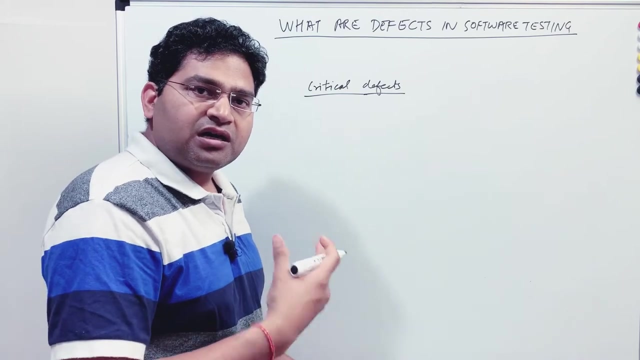 remember about the defects. when during the test execution phase is basically the say, for example, critical defect percentage, right, So critical defect. I'll explain what critical defects are. So critical defects say for example: okay, when we say critical defect, these are the defects which block the testing or they are the 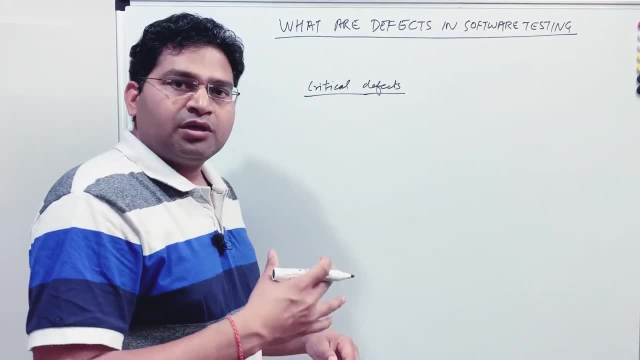 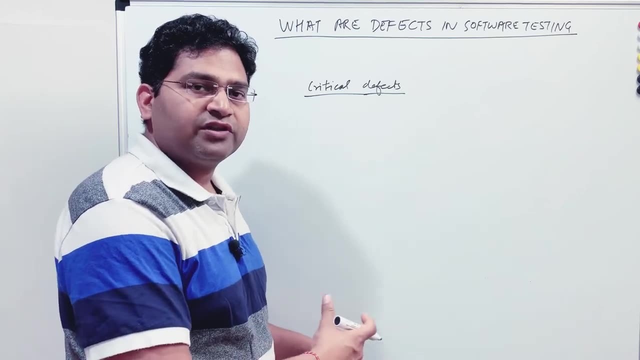 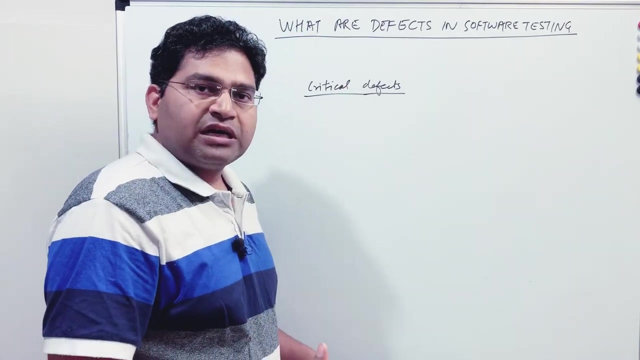 defects which will have the maximum negative impact on the business, or they will have negative impact on the actual processing of the software or the functionality of the software. Any such defect which will have the major impact or either on the revenue or the business are categorized as: 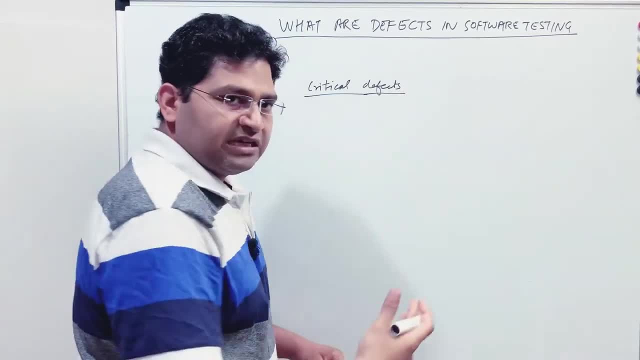 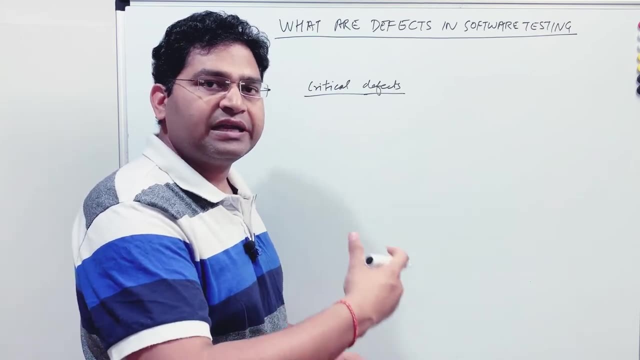 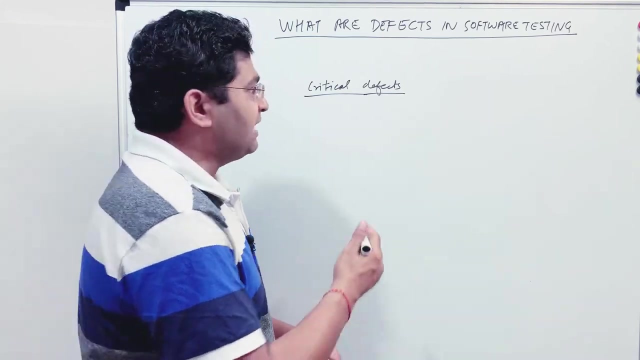 a critical defect. So, for example, this login functionality right. So login functionality. if it is not working, then how will a user go ahead and log in and place the order? They can do it as guest, but this is one of the key functionality that needs to be fixed. So 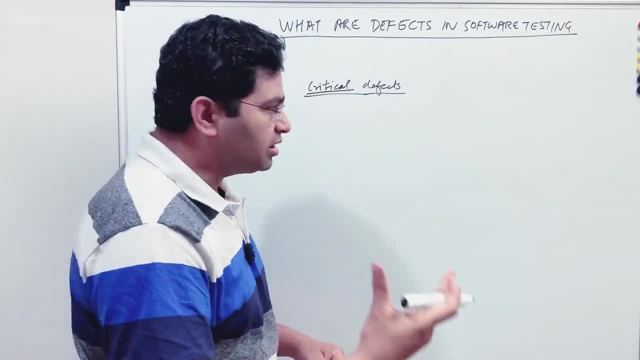 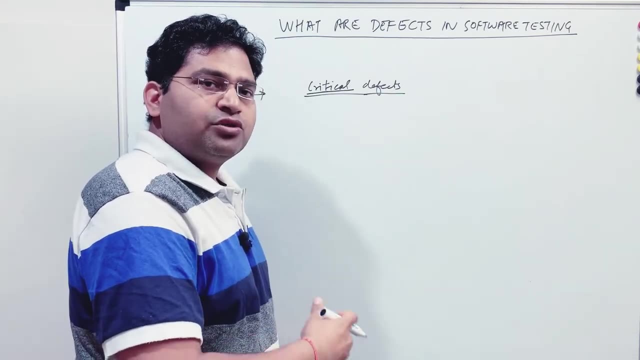 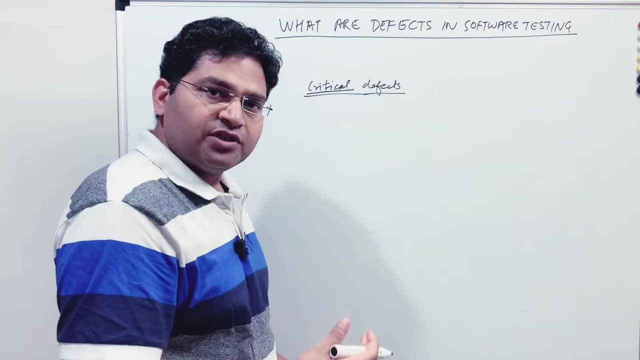 if login functionality of the website is not working, then that defect can be categorized as critical defect. And when you are doing the testing and during the testing phase, when you are finding the defect, as a test manager or test lead you come up with some of 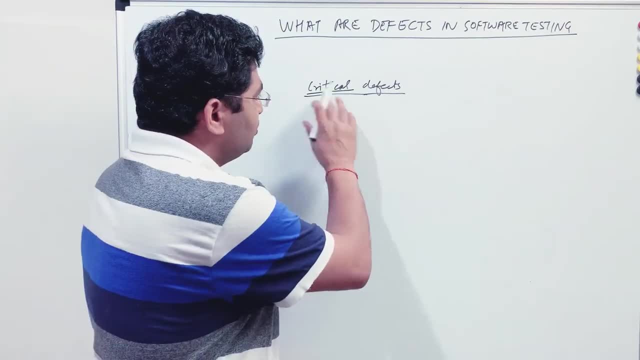 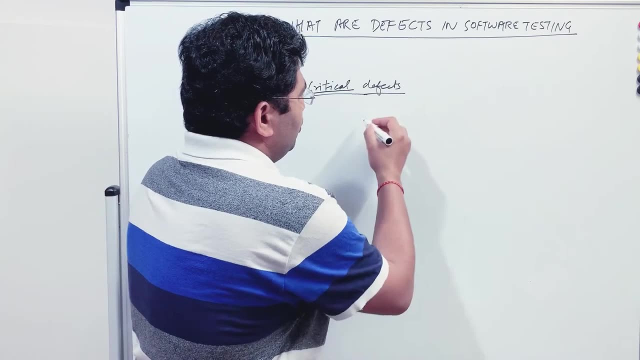 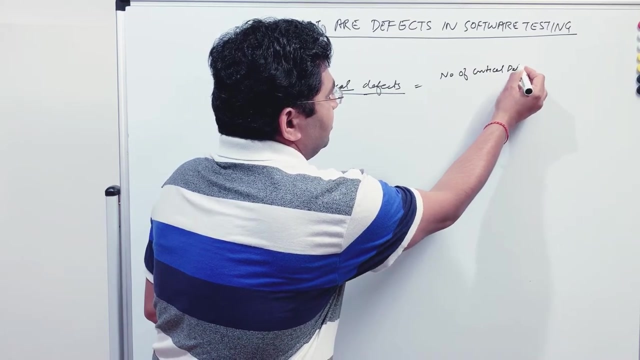 the test metrics or the defect metrics. So the first one is basically, you know, critical defect percentage. So how you find these metrics, So whatever number of defects you have found, say, for example, number of critical, critical defects. Okay, So during a particular testing phase, number of critical defects that you find upon. total number of defects, So total number of defects during that phase in 200.. So that's what your critical defect percentage is. Now, if this critical defect percentage is high, then that means there are lots and lots of critical defects within the application. So 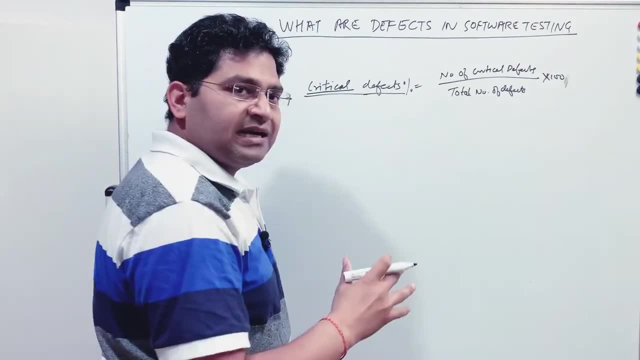 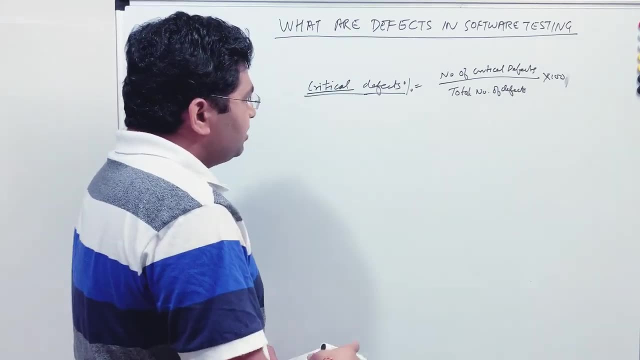 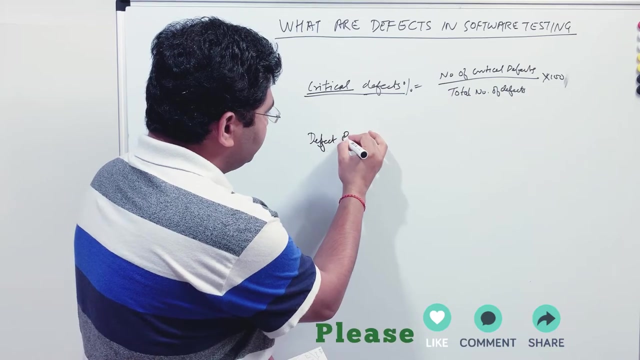 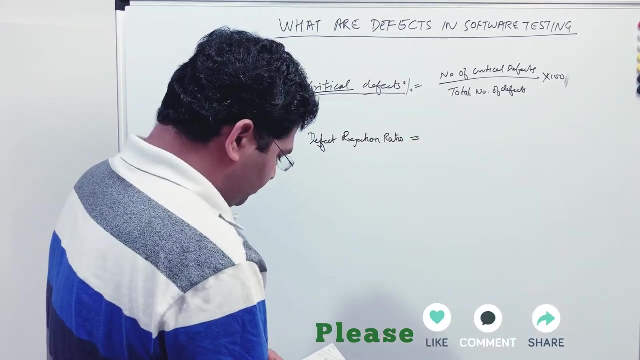 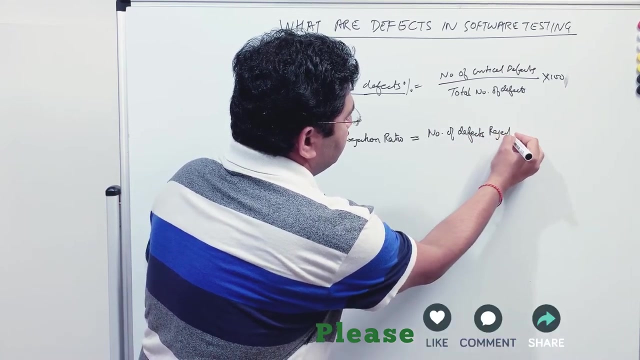 this metric helps you to understand what is the code quality or the work that has been done as part of the development. The another important metrics is defect rejection ratio. Okay, So defect rejection ratio. Now. defect rejection ratio is number of defects rejected and upon total. 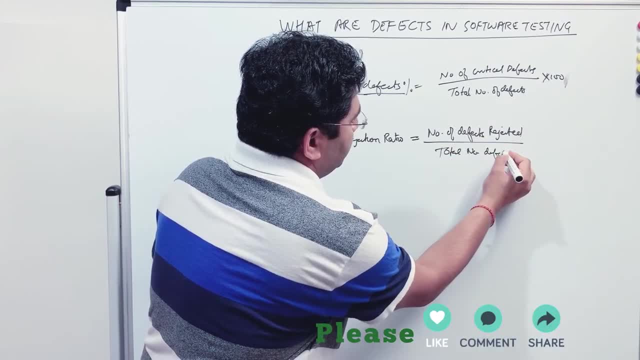 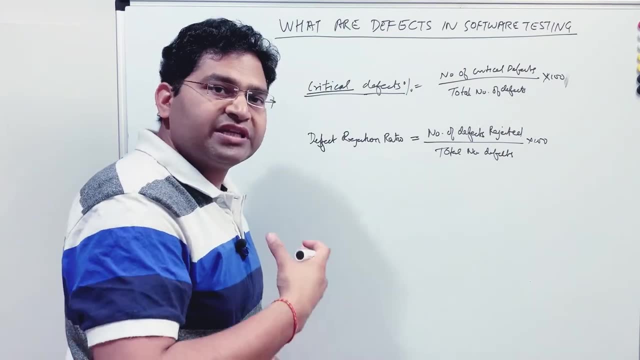 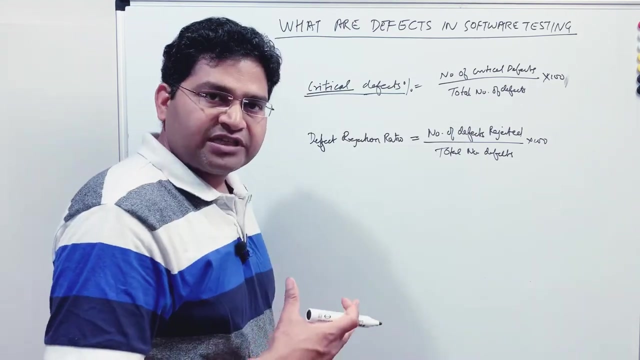 number of defects And the product is divided into 100, okay, so defect rejection ratio: how many defects have been rejected? so, as a testing teams, if we have five people in the testing team and people are raising the defect as soon as they are analyzing the defect and they think that it is a defect Once the 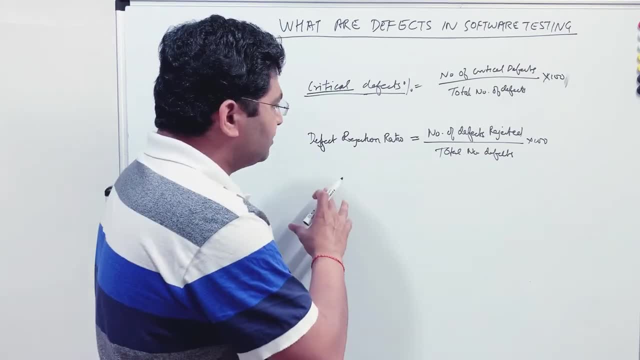 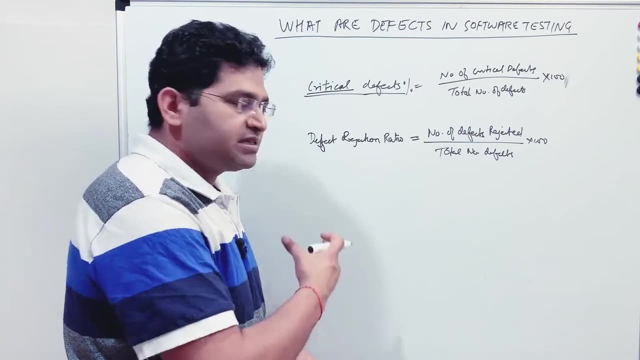 defect has been raised and analyzed by the dev team and they found that the defect is not because of the code or it's some issue because of the data that has been used by the test team and they reject the defect that this is not the actual fix. 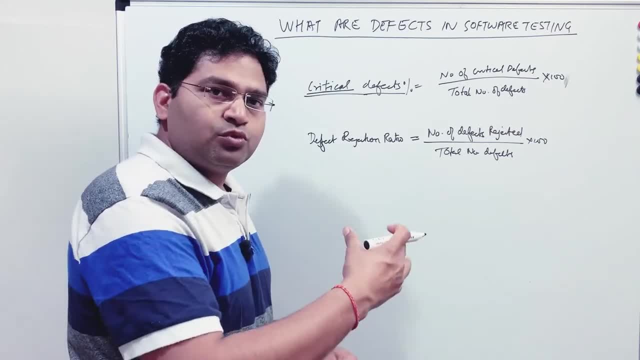 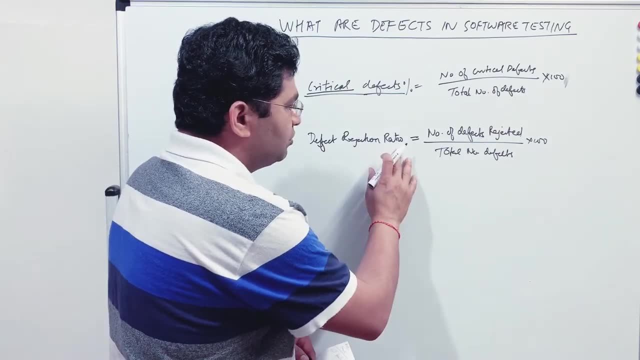 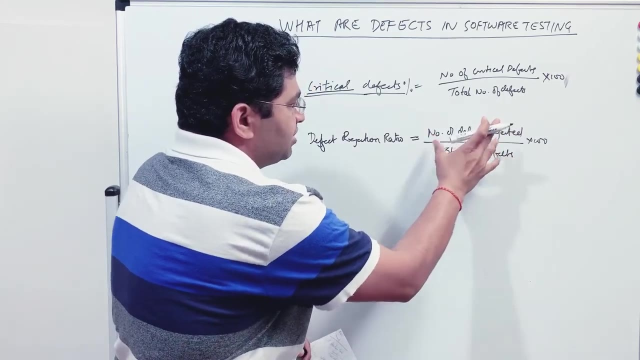 that they need to do. you need to follow certain steps to test that particular bit. in that particular case, the defects will get rejected. so what this defect rejection ratio will do is number of defects that got rejected in a particular cycle or a particular phase. you have those numbers here, so for 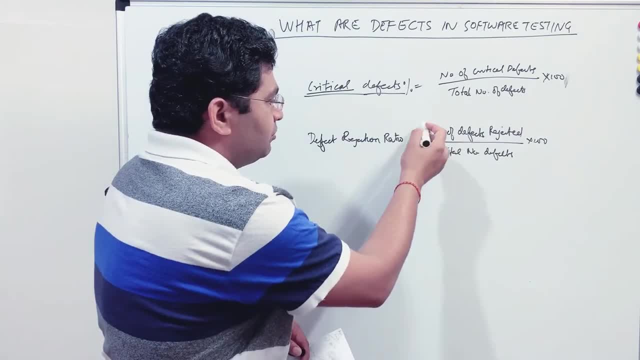 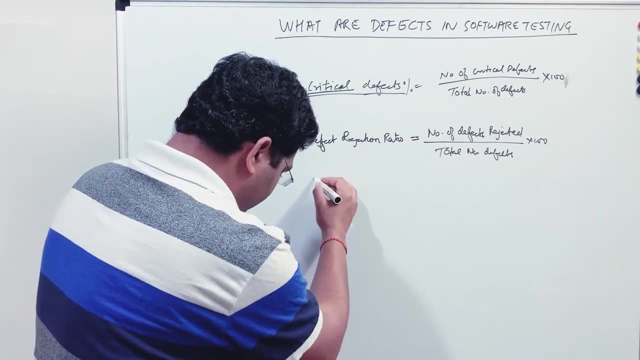 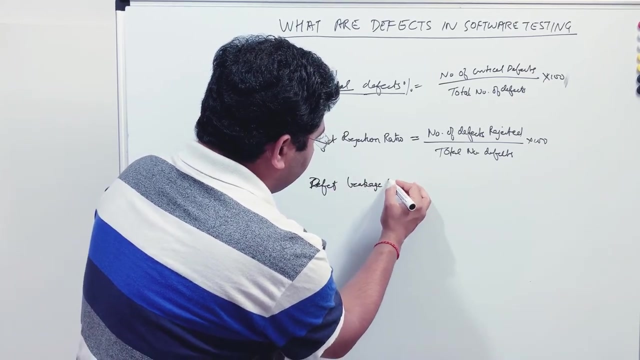 example, 10 defects got rejected out of total hundred. so you get a defect rejection ratio in that particular context now, defect rejection ratio, and the other one is defect leakage ratio. okay, defect leakage ratio is also very important matrix, and what defect leakage ratio shows you is so in the leakage. 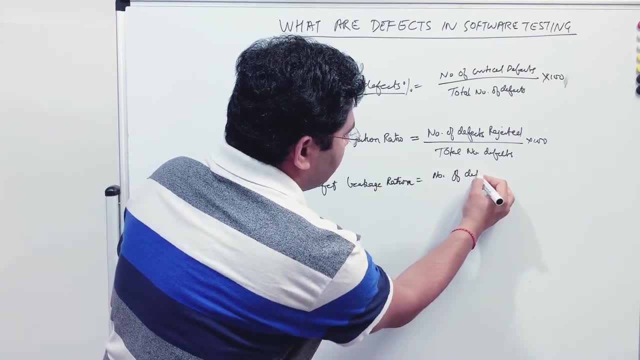 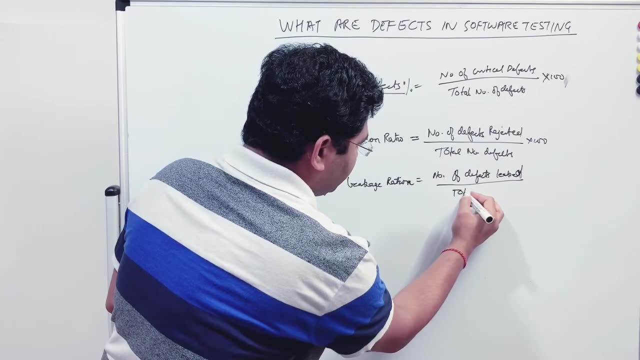 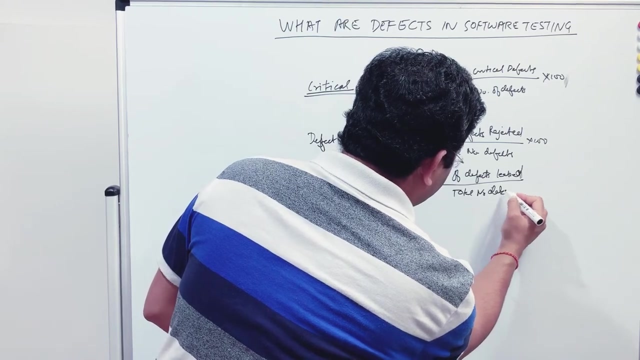 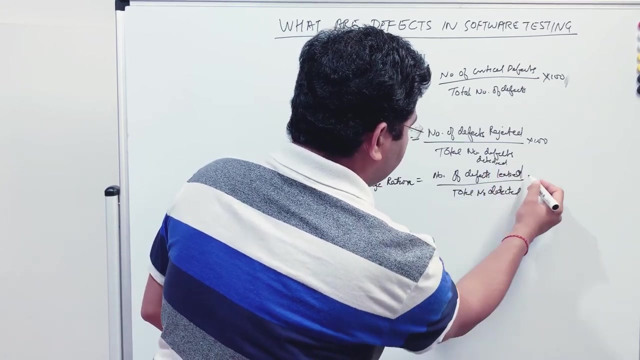 ratio, a number of defects. let me write it first. so number of defects leaked, and upon total number of defects: total number of defects, total number detected. okay, total number of defects detected here, so detected in that particular phase. total number of number of defects detected into hundred, right. so defect leakage ratio. so, for example, 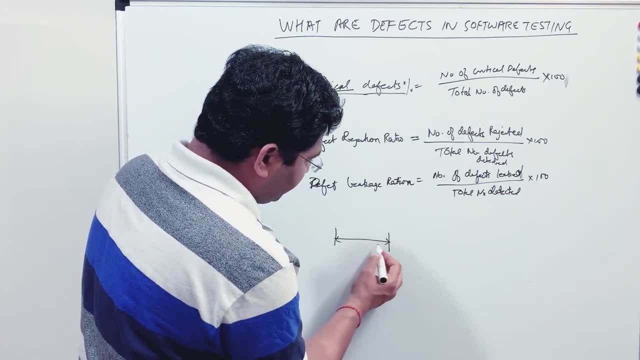 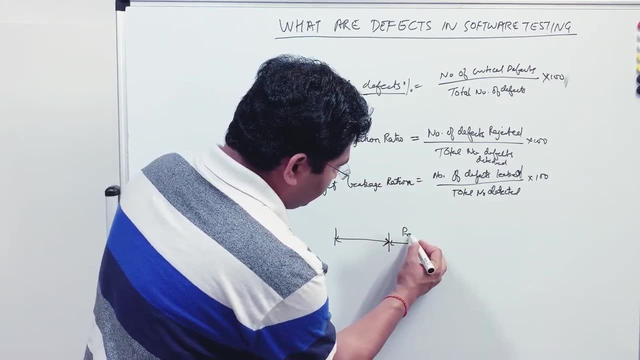 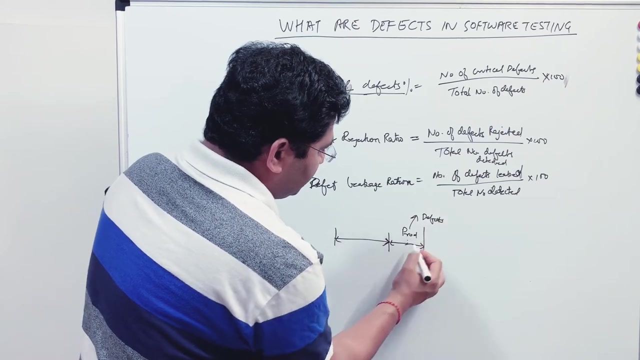 you have a testing phase and after testing phase, the the application being deployed into the production. okay, so in the product. so once your application is in the production, how many defects are being found here? okay, say, for example, after the production deployment there were 10 defects that were found in the production deployment. 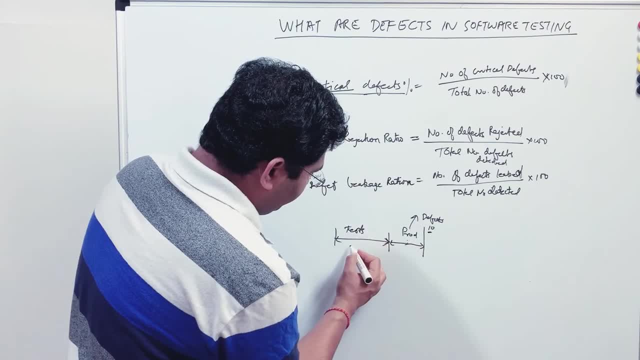 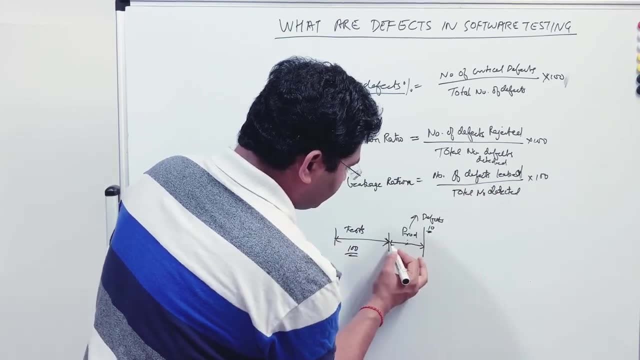 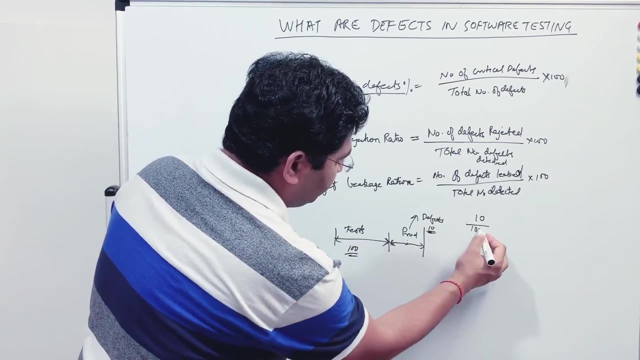 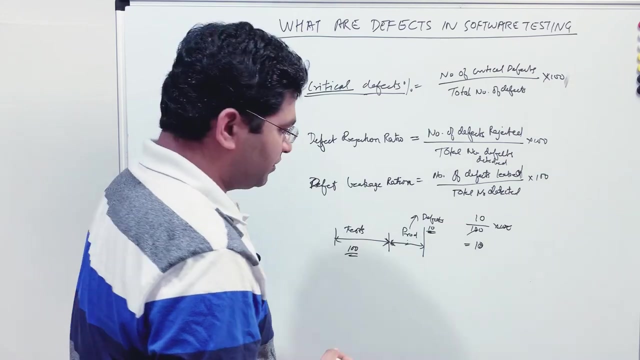 and in the actual test phase you found hundred defect, right? so defect leakage ratio is basically number of defects leaked. so in the production there were 10 defects that were found and total defects that were detected in the test phase was 100 into 100, right? so the ratio of leakage is 10 percent. okay, this number and 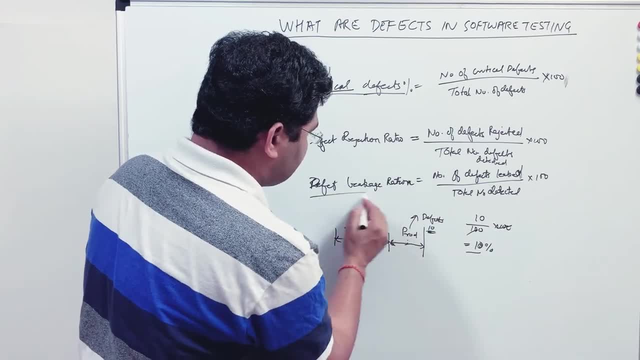 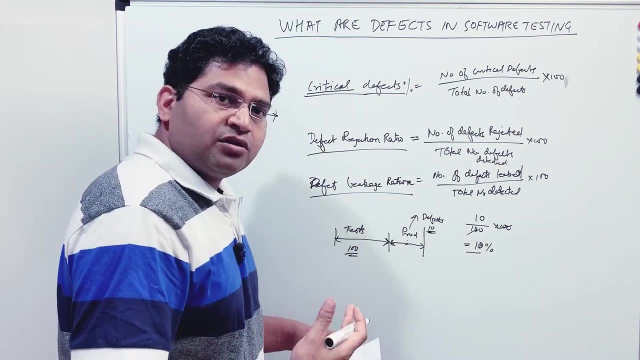 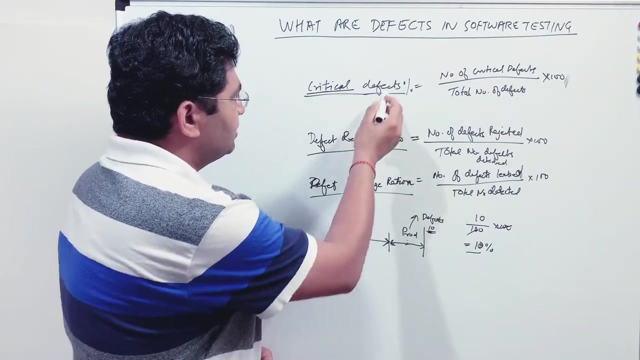 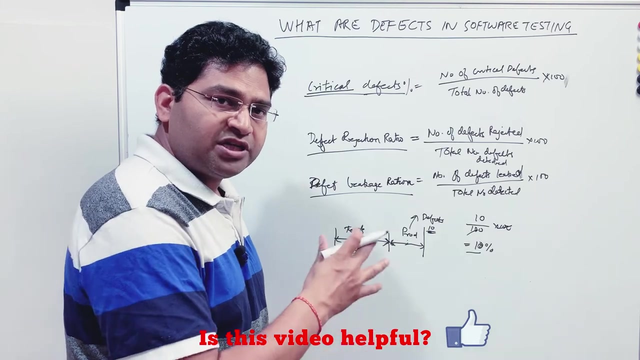 rejection ratio number. so defect leakage ratio and defect rejection ratio should be as low as possible. this shows the effectiveness of your testing activities right. so these metrics are really important. defect rejection ratio. critical defects. there are many other metrics that you can use. you can google and find out the different metrics, but these are the critical, critical ones. defect.